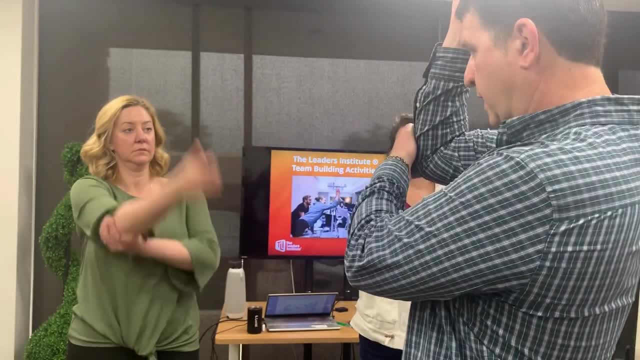 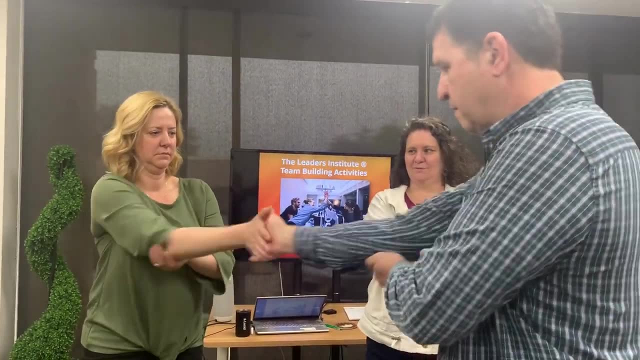 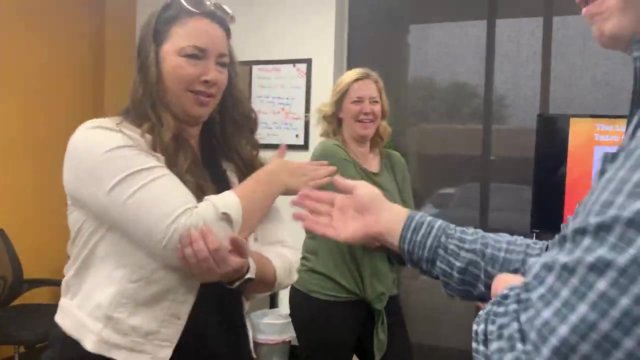 For instance, if you started with a high five, you know, do a high five and then a low five And then a high five. After you've shown the group that addition, have them. Have them use the new version of the handshake for four people as well. 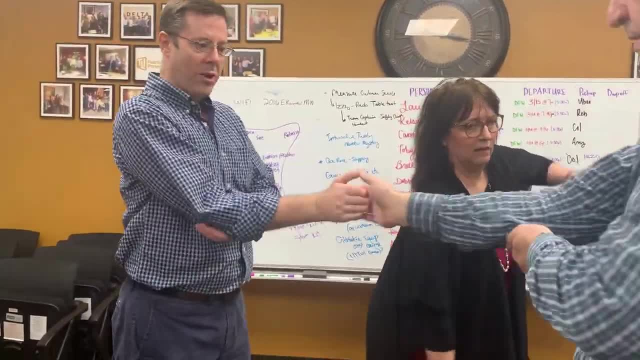 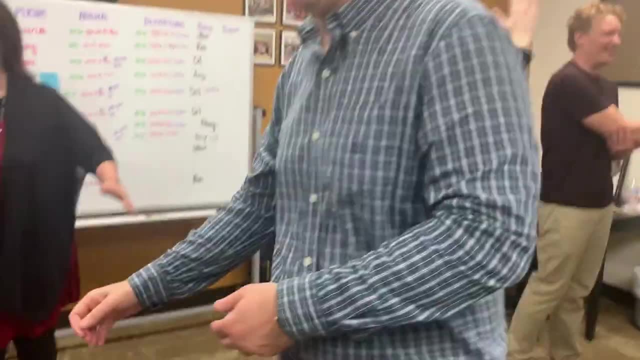 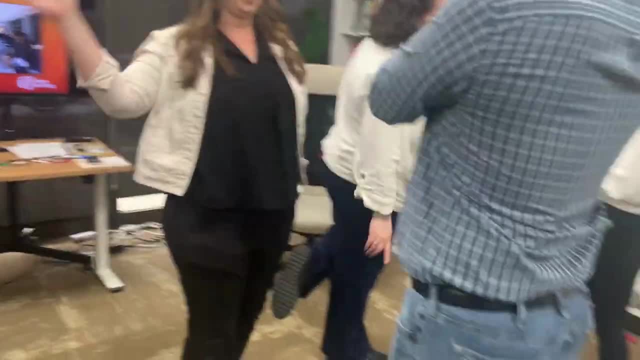 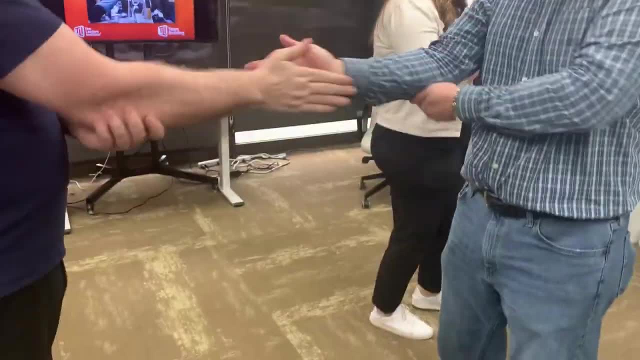 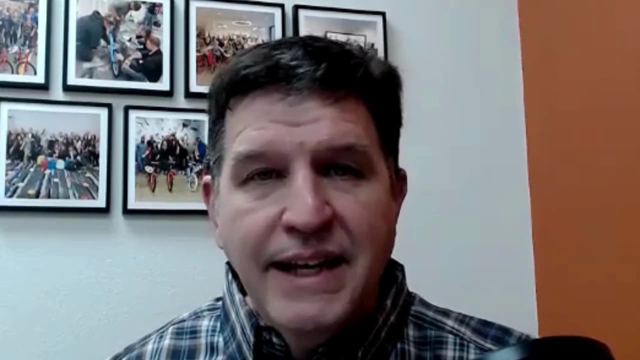 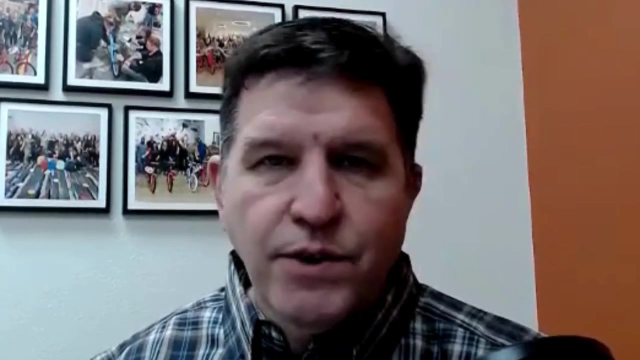 By the way, this activity is a great way to get the people in the meeting up and moving around. So here are three really easy ways to kind of use the secret handshake in your meeting for a specific purpose. Now, obviously the easiest. the first one is just as an icebreaker to start a meeting. 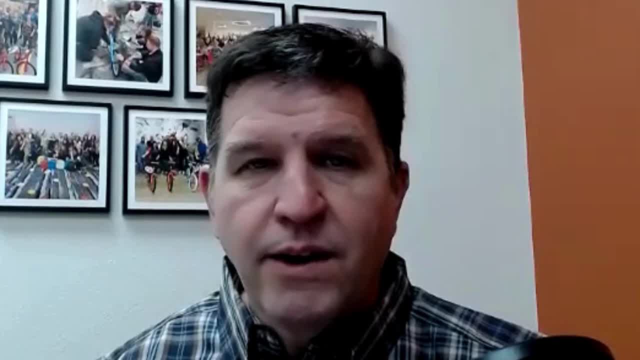 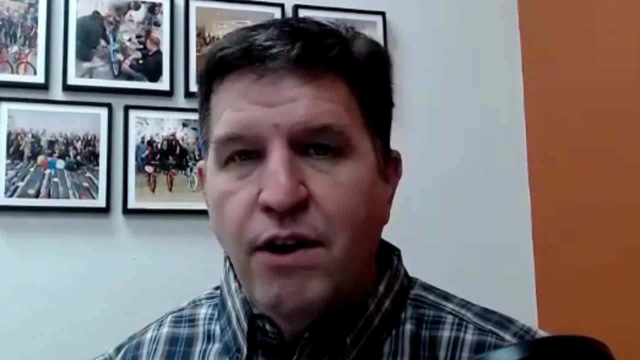 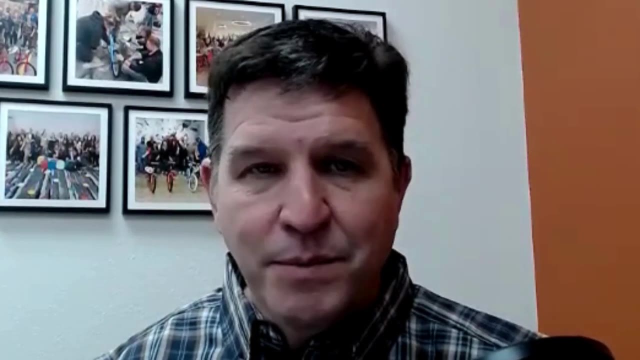 That it's really helpful. It helps to get kind of a stoic crowd or a quiet crowd to more freely participate in the meeting. You're basically giving them permission to interact with each other and talk during the meeting. The second thing that you can use this for, though, is that you can use it as a way to kind of mix up the tables in your meeting. 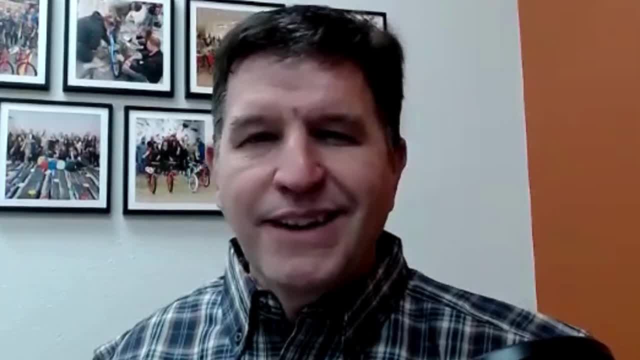 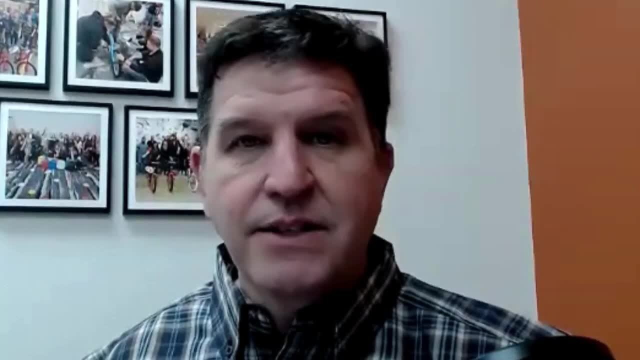 So if you, most of the time when people enter a meeting room, they're going to sit at the table with people that they know best- It could be their friends- or if it's folks that just met each other, a lot of times they're going to sit next to the person that they just met. 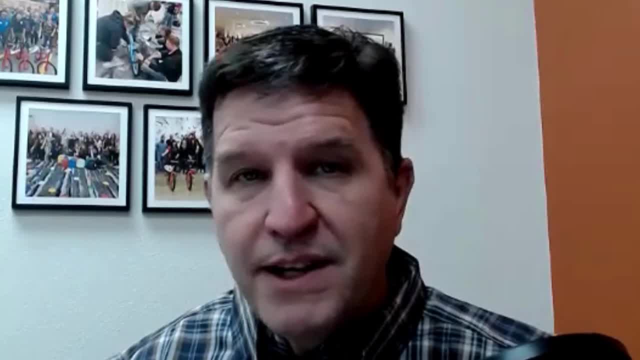 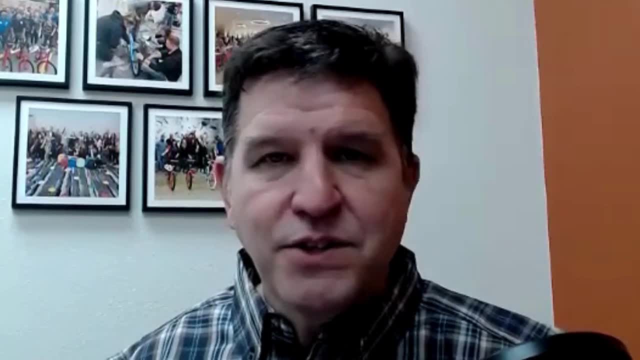 So, basically, if you start the meeting with the secret handshake, after they move around the room they're going to be in a totally different spot than where they started. So just have them sit down at the chair that's closest to them when the activity finishes. 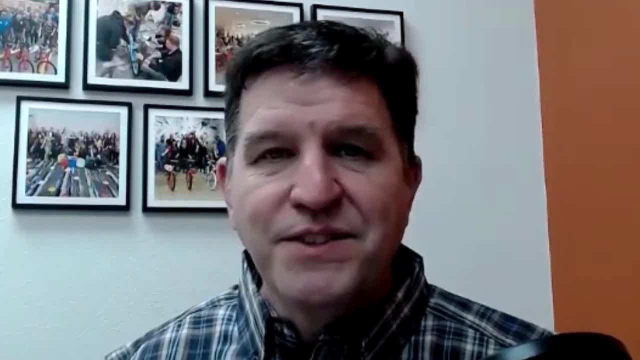 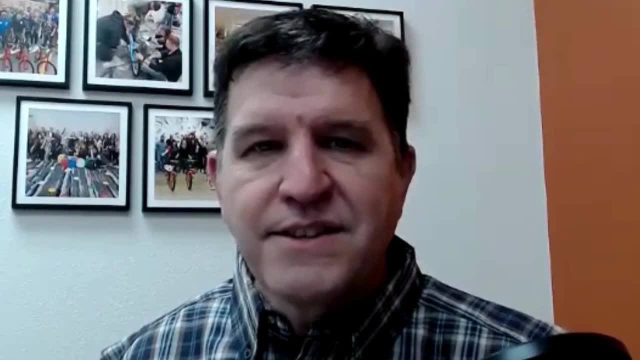 You got the teams all mixed up. A third way that you can kind of use this- and this is a really fun way to kind of add a competition to the meeting- So after the groups practice that final crazy handshake, give them 60 seconds or so.